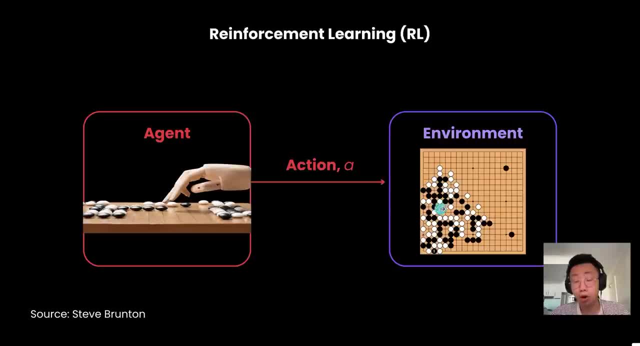 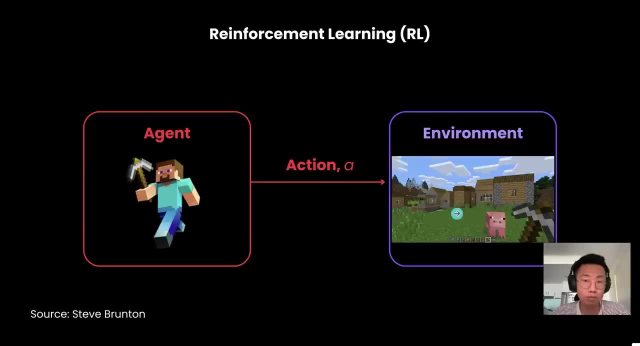 in a maze try to find a way out, as well as games like chess and go, And the agent is able to take actions in this environment. In video game scenario, it will be moved from point A to point B and chess and go will be. 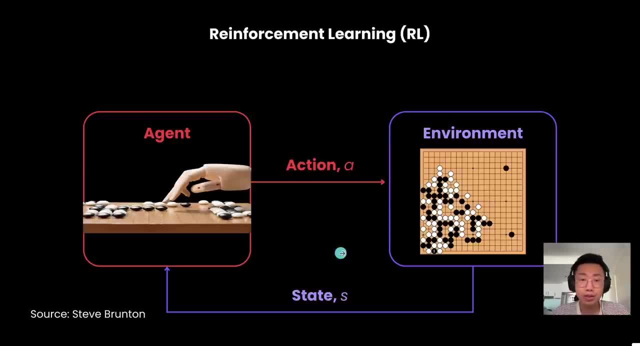 placed and moved on the board And after agent taken action, the agent will be a new state which can be a new chess board after agent made a move And on the other hand there can also be rewards or penalty signal back to agent. 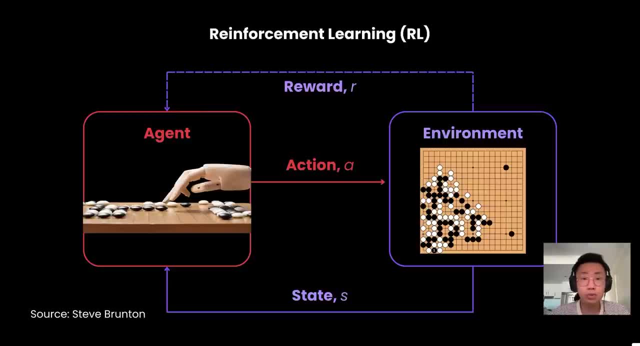 So the agent can know whether the action I take is contributing to the goal or not. And the agent will repeat this process for multiple times. And really the goal of a reinforced learning system is developing a strategy to decide which action I should take in a given state that can maximize the total amount of future. 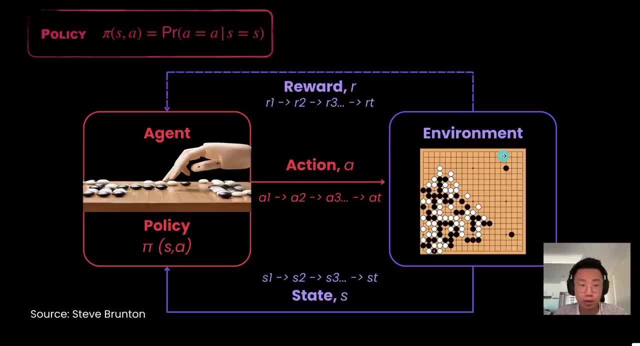 rewards that I can possibly get, And that decision making engine is what we call policy network, So it is pretty confusing term policy, but what it really is it is basically a function where it can tell you, based on the state, that agent is taking. 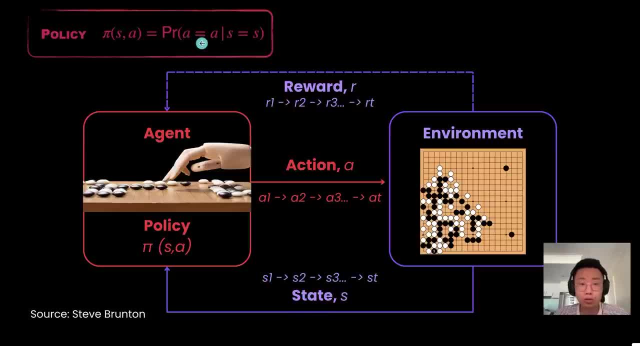 Now, which is S how likely the agent is going to take a certain action. And one of the most tricky part of reinforced learning is a reward, Because in many scenarios the agent won't get any immediate reward or feedback after taking action. in chess or goal example, you will only know whether 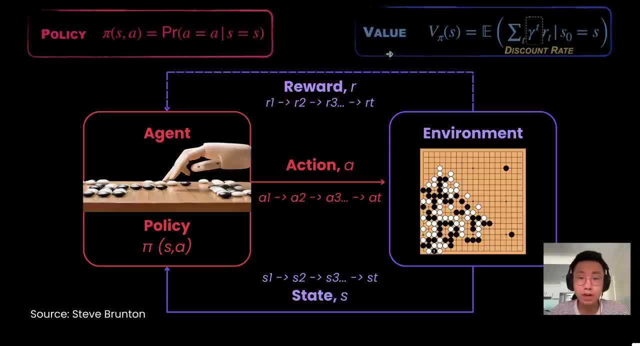 you win after the game finish. and this is where the second part, value network, comes in. It is another AI that help you evaluate what is the total amount of future rewards If the agent take a certain action. So at high level there's a policy network who is proposing the action that agent can take at a given situation. 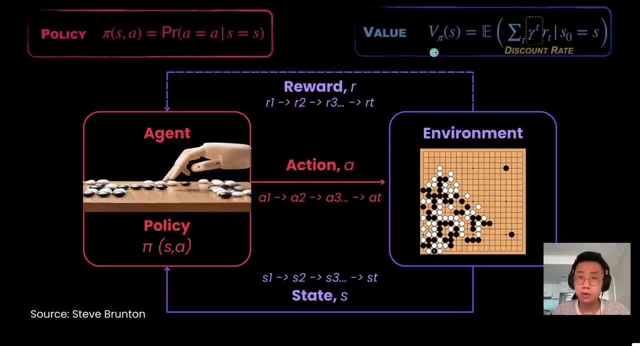 And there's a value action that can estimate the value of all those proposed actions And they kind of reinforce each other. So at the beginning the agent has a pretty poorly defined policy and all the action they take can be quite random. After each game, the value network can improve its estimation based on the actual results. 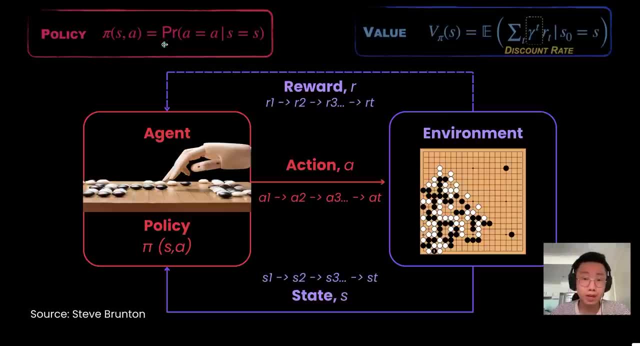 And the policy network can use that to improve its decision making quality. So this is high level. what a reinforced learning system. If you want to Learn more, I would recommend to go watch Steve Burton's video. He has lots of deep dive into the reinforced learning space. but once the system is done, 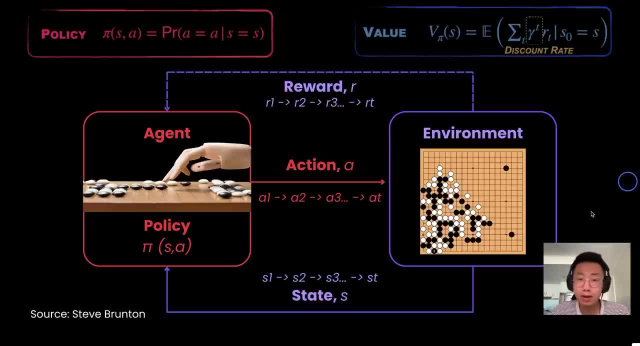 it is extremely powerful because it is able to just self play and try thousands or even millions of different variations to complete the goal, from which process the agent is able to discover new methods or new strategy that no one has ever found before, And the best way to look at it is some past projects from DeepMind, which is 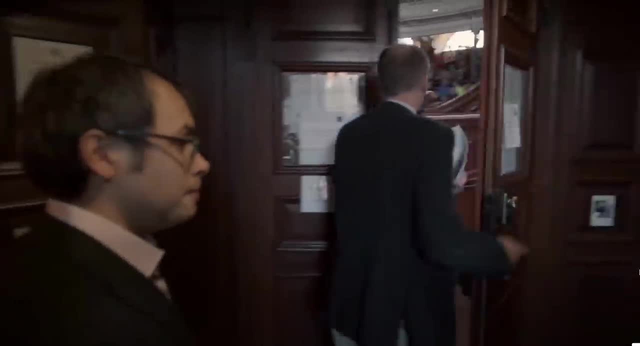 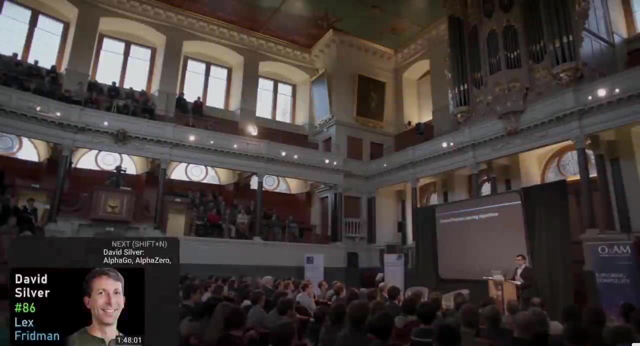 institution that developed AlphaGo. So this is back 2012, when DeepMind firstly showcased a few examples of how AI is exceeding human level performance in certain tasks. So I'm going to show you a few videos of the agent system, the AI. 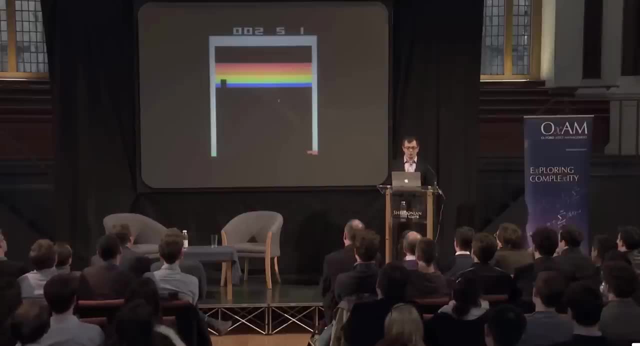 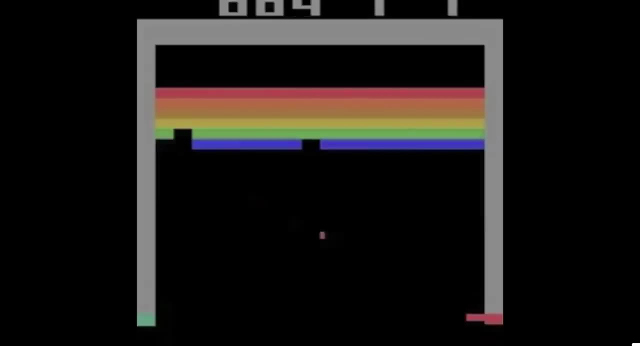 So let's start off with breakout. So here you control the baton ball and you're trying to break through this rainbow colored wall. The agent system has to learn everything for itself just from the raw pixels, doesn't know what it's controlling, doesn't even know what the object of the game is at the beginning. 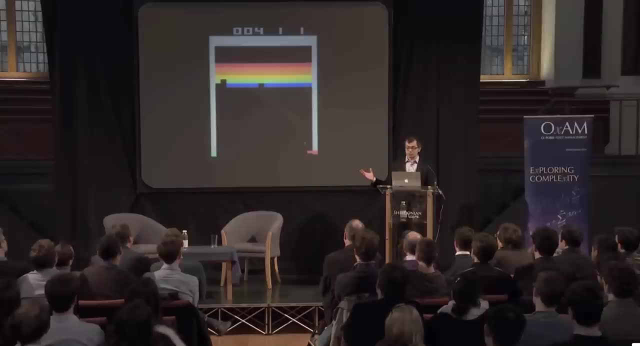 After a hundred games You can see the agent is not very good. It's missing the ball most of the time, but it's starting to get the hang of the idea that the bat should go towards the ball. Now, after 300 games, it's about as good as any human can play this and pretty much gets the ball back every time. 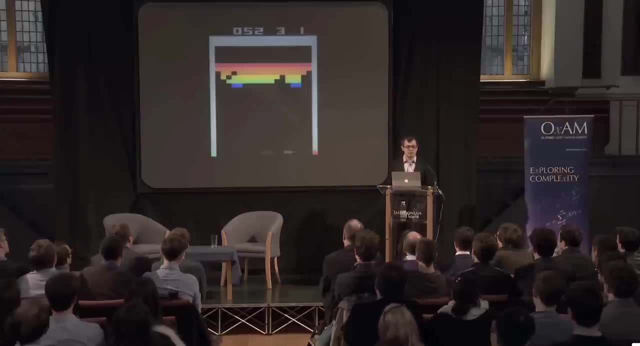 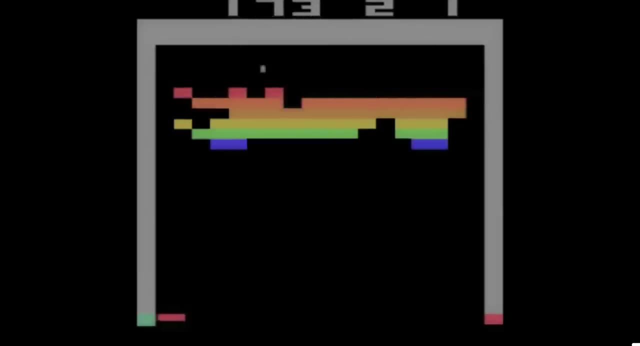 We thought, well, that's pretty cool. but we left the system playing for another 200 games and it did this amazing thing. It found the optimal strategy was to dig a tunnel around the side and put the ball around the back of the wall. 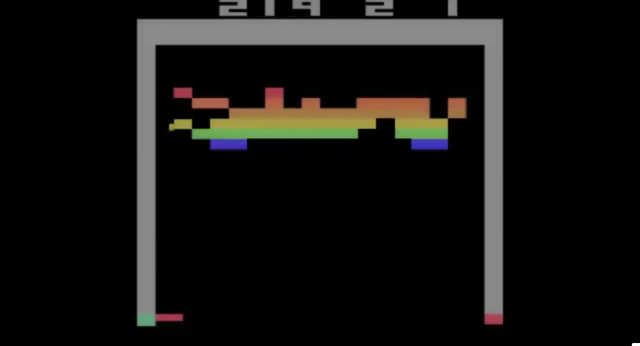 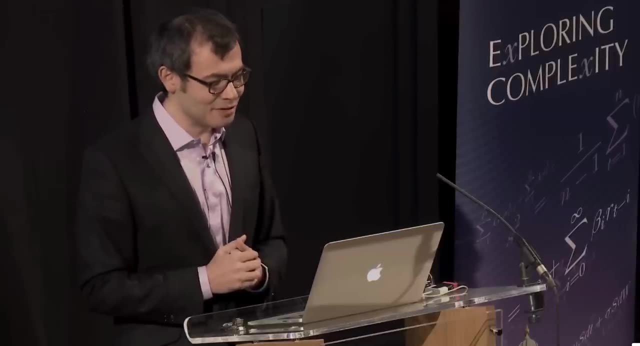 The researchers working on this, amazing AI developers, but they're not so good, So good at breakouts and they didn't know about that strategy. So they learned something from their own system, which is, uh, you know, pretty funny and quite instructive. 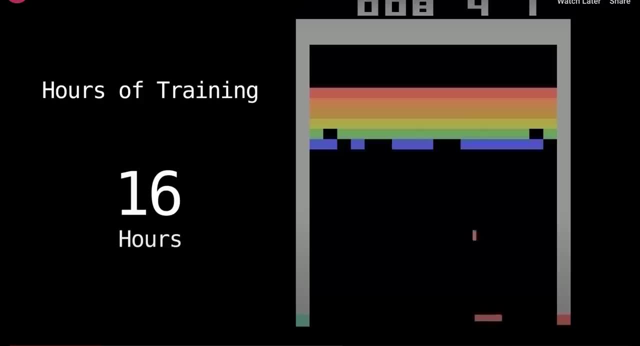 I think about, uh, the potential for general AI. So, through reinforced learning agent, not only get to a point where it can play the game well, but also develop a strategy. that is not very obvious for many people, because it is able to explore a wide range of different paths that has never been taken before. 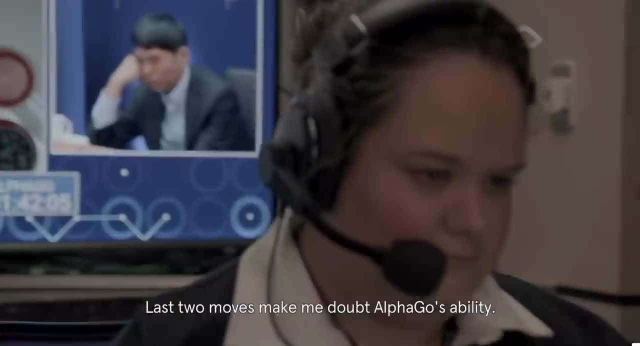 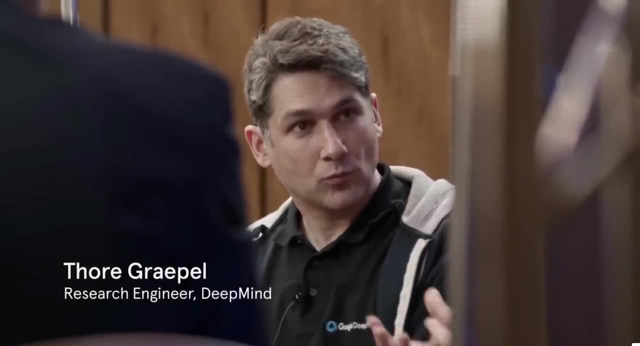 And a few years after they introduced AlphaGo, which is a great example where it showcased AI can explore strategy. Yeah, We're never explored before. Can you sort of share a bit of what is going on in AlphaGo? So, uh, AlphaGo has these three main components. 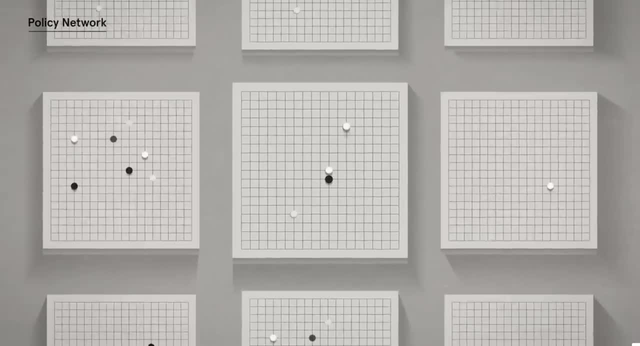 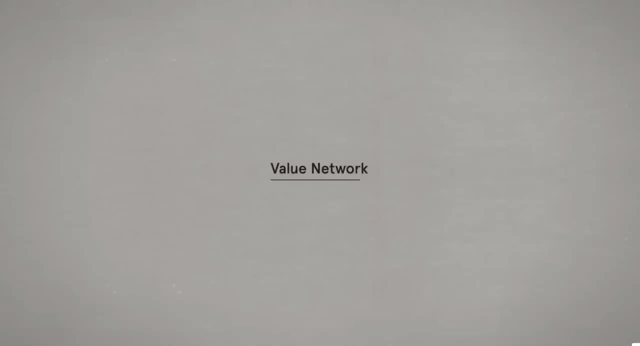 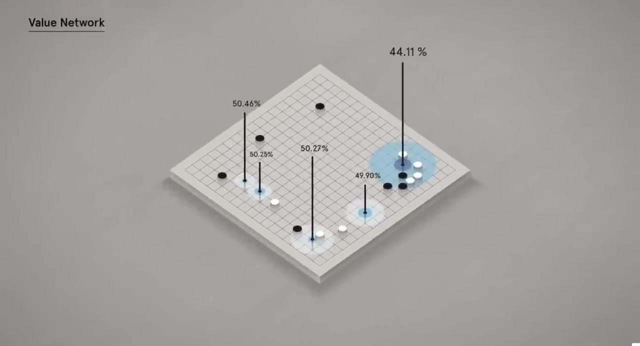 There's the policy network, which was trained on high level games to imitate those players. And then we have a second component, We call this the value net, and it can evaluate the board position and say what is the probability of winning in this particular position. 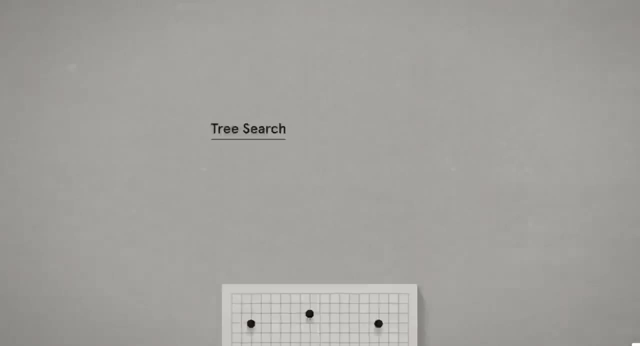 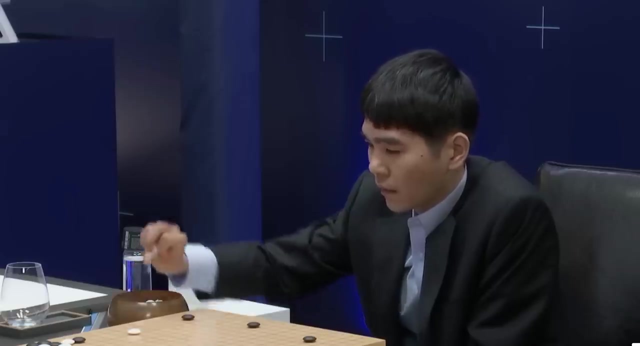 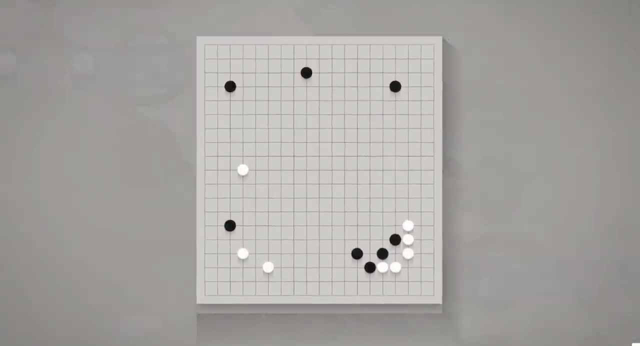 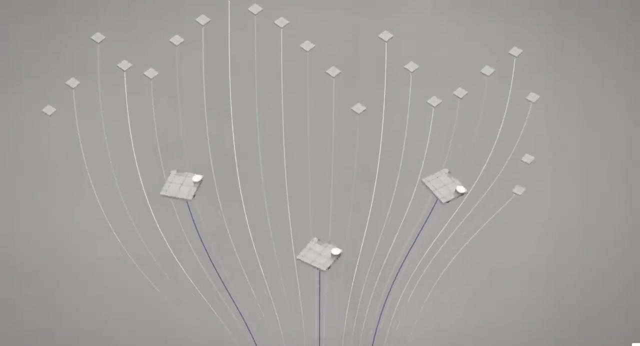 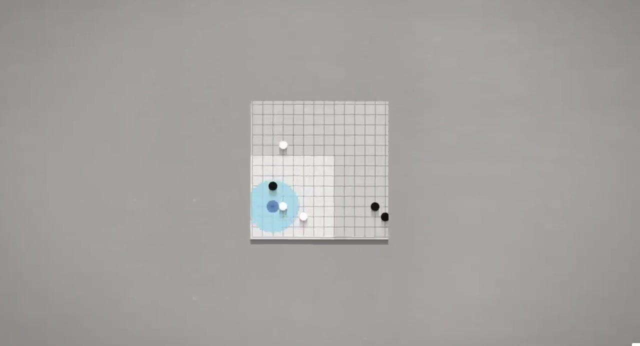 And that third component is the tree, And it can do a lot of research where it would look through different variations of the game and try to figure out what will happen in the future. take a position like this: first, the policy network would scan the position and come up with what would be the interesting spots to play, and it builds up a tree of variations and then employs this value net that tells it how promising is the outcome of this particular position. 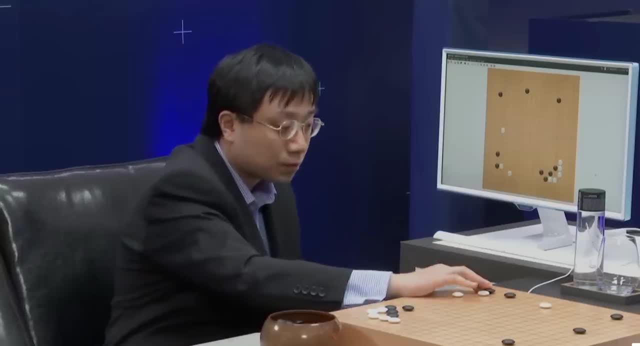 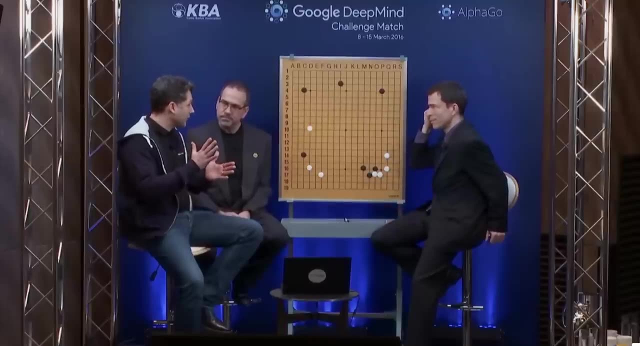 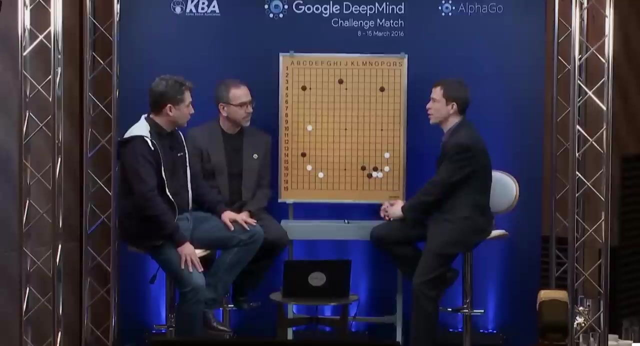 So AlphaGo tries to maximize its probability of winning, but it doesn't care at all about the margin by which it wins. Okay, So when you see a slow looking move, that's maybe an indication that AlphaGo thinks it has a good chance to win. 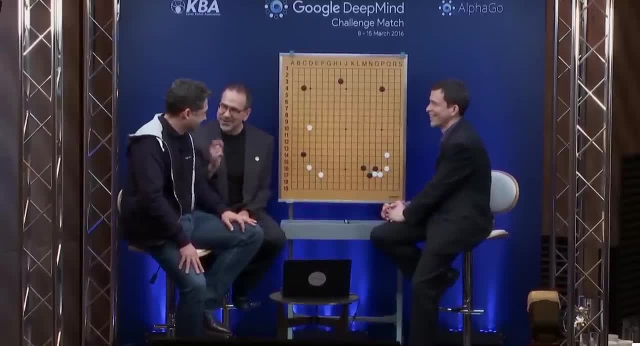 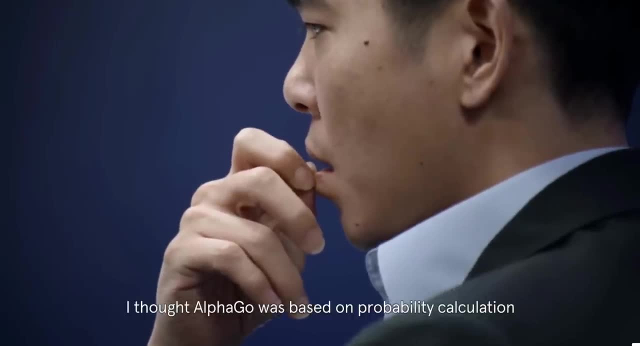 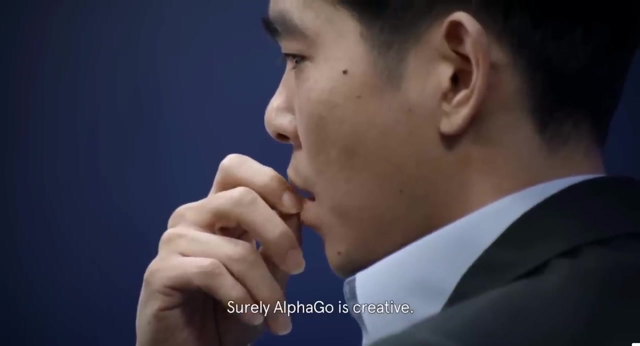 Yeah, that that is a little giveaway. And with this system set up, AlphaGo not only are able to make quality bets on every single move, But also able to discover and create new strategy that were never discovered before. And here were a few example where AlphaGo initially made a move that no one really understood. 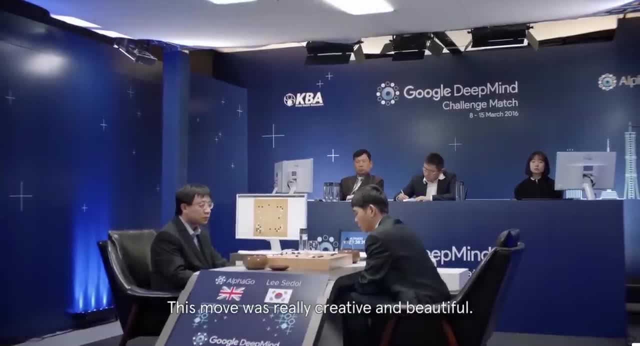 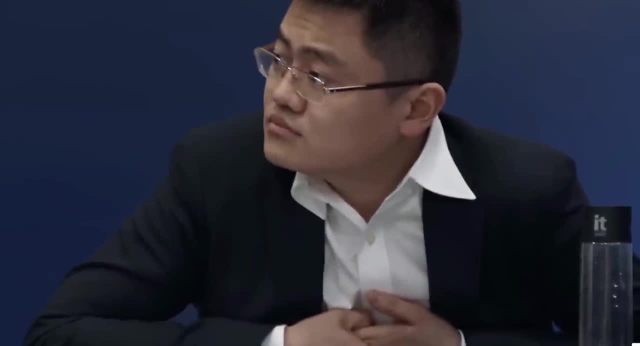 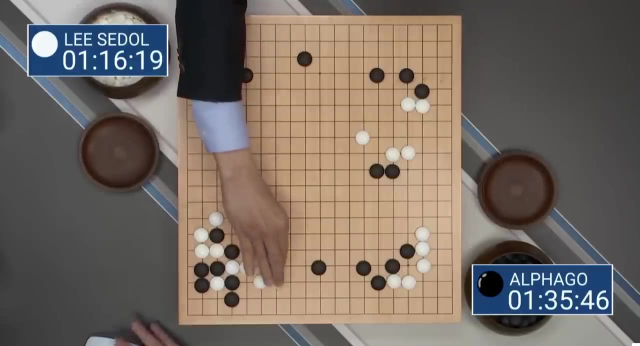 It looks bad but turned out to be a critical move for a super long-term strategy. The more I see this move, I feel something changed. Maybe for human we think it's bad, but for AlphaGo, why not? Go is like geopolitics, like something small that happens. 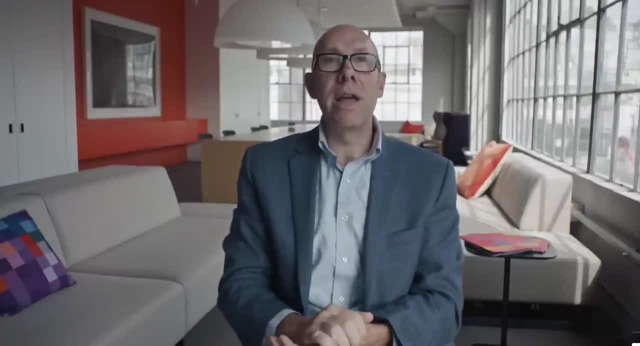 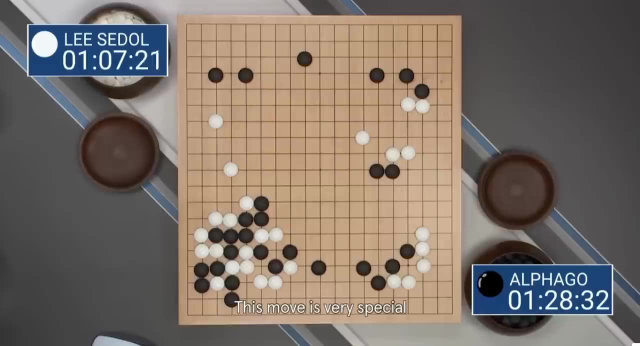 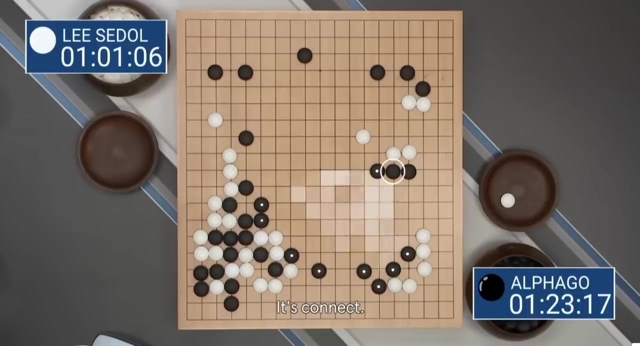 Here they'd have a ripple effect. you know, hours down down the road, in a different part of the board, the game kind of turned on its axis at that moment. This move is very special because with this move all the stones played before is work together, is connect, is look like a network, link everywhere. 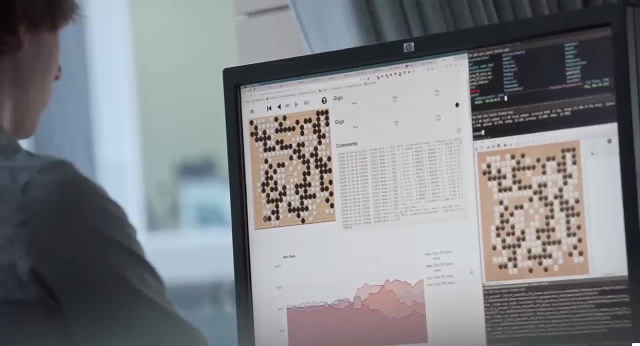 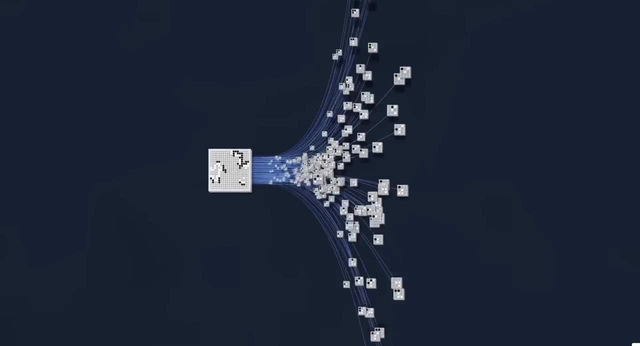 It's very special, very special. This is an effect where AI can explore all sorts of moves and discover new strategy that were never discovered before. It's special, It's super exciting. But what does this really mean for large-large model NGPT? 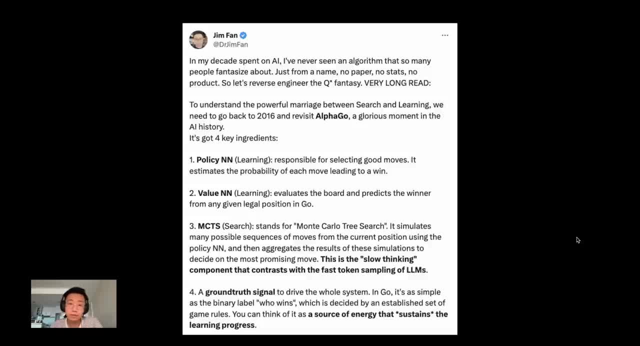 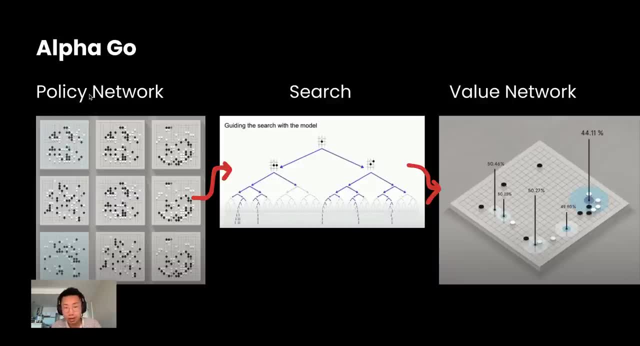 One hypothesis is from Jim Fan, who is a senior AI scientist from NVIDIA. So the way AlphaGo works is the use policy network- which, if you remember, it is actual decision-making AI- to propose what are probable moves. So they use policy network to narrow down a list of high quality moves so that the AI can narrow down and play out a few steps ahead and understanding the ripple down effects of winning and losing. So the way AlphaGo works is the use policy network to narrow down a list of high quality moves so that the AI can narrow down and play out a few steps ahead and understanding the ripple down effects of winning and losing For all those high quality options. 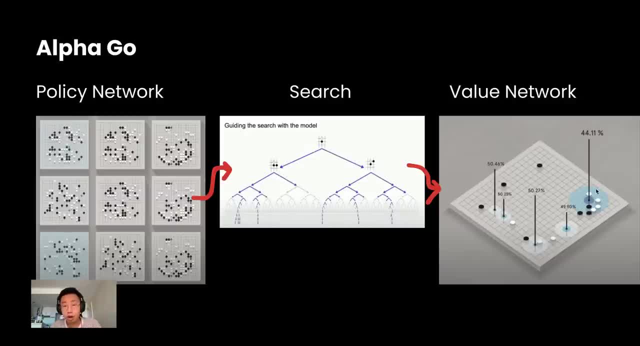 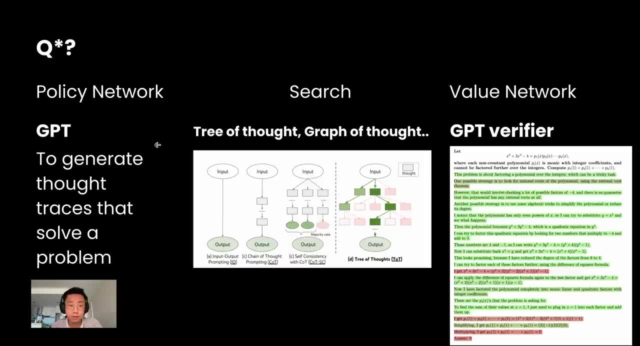 And, as a result, return back an estimated value for each options to understand which one is the best move, significantly improve the results and whether that can be the same architecture for the skill star. So policy network is basically a GPT that is really good at posing what are the good potential paths to solve a given problem. 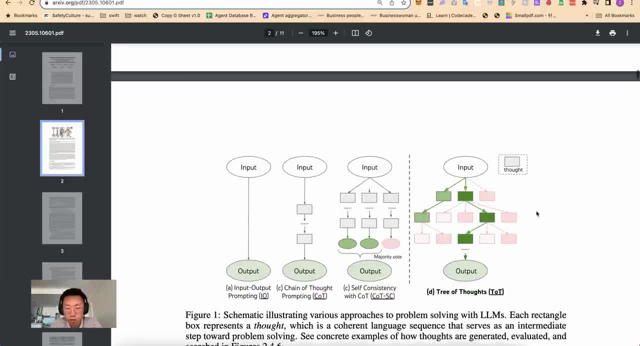 And then it can use methodologies like trade-off thoughts, which is one of the prompting methods that has shown significant better performance compared with other methods. And then it can use methodologies like trade-off thoughts, which is one of the prompting methods that has shown significant better performance compared with other methods. 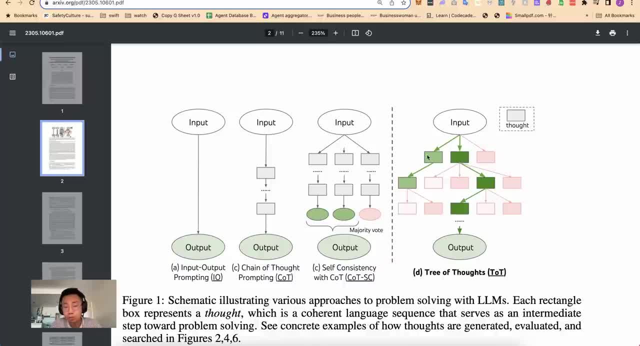 And then it can use methodologies like trade-off thoughts, which is one of the prompting methods that has shown significant better performance compared with other methods. Basically ask large language model to propose a number of different ways of how a problem can be solved, as well as number of steps for high quality candidate. 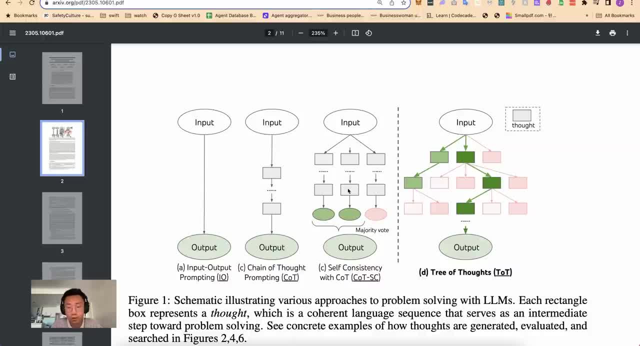 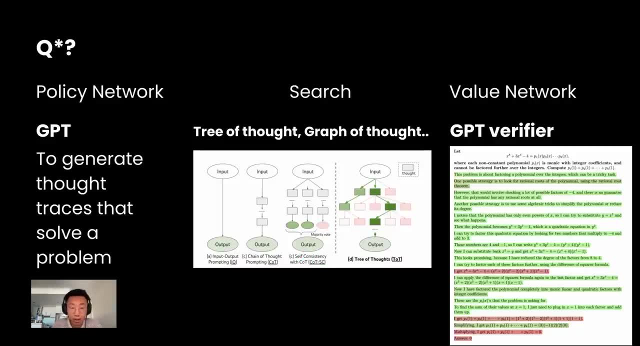 And so far this method hasn't been really widely adopted, And one of the reason is that it costs a lot more money and it's a lot slower. But it's possible that open AI figure out a more efficient way for large language model to search for the optimal path. 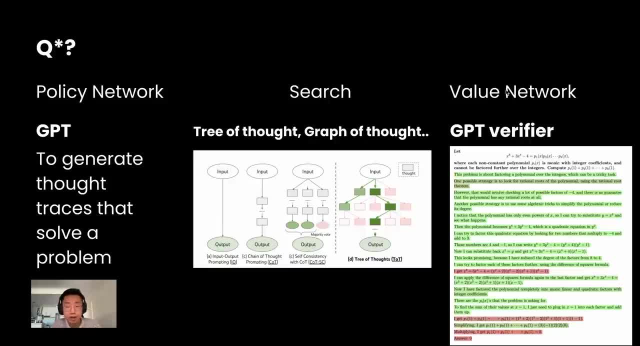 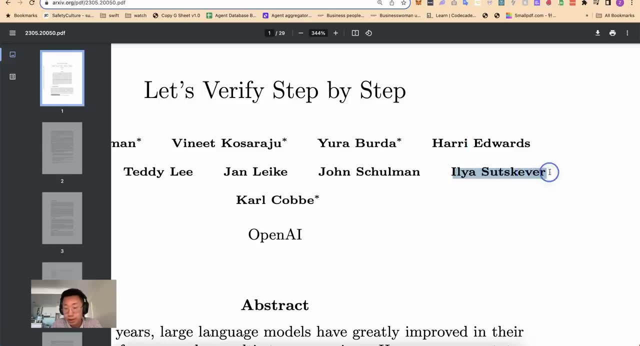 And in the end there could be another GPT- play the role of value network which can review the thoughts of large language model And provide feedback and critique of how large language model's reasoning and logic should be improved. here- And this is from a research paper published by open AI called let's verify step by step, where Ilya is also the author- 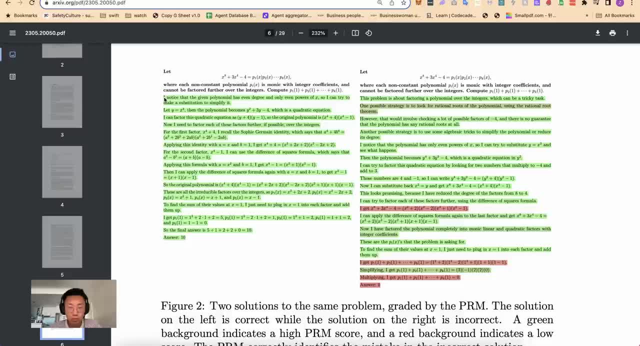 They explore implementing the reward model where they basically ask large language model one to solve a math problem with chain of thought methods, where it will display every single step about how he thinks the problem can be solved, And then get a large language model to review and critique each reasoning step, which is quite different methods of how to solve a math problem. 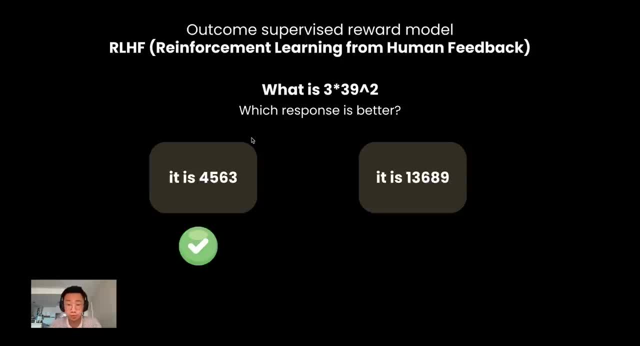 They also study how reinforced learning is currently adopted today for large language model. So far, the common methods is called reinforced learning from human feedback. It basically asks a large language model to generate a few different answers for a given task and then let a human to compare and choose which one is better, which is more outcome-based. 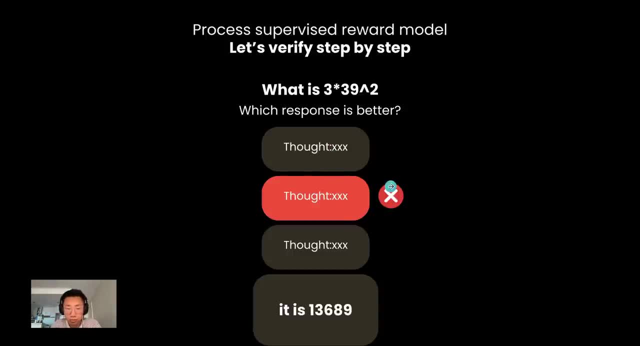 Versus. let's verify step by step where they get another large knowledge model to review the actual thinking process of the original large language model that leads to the final results And give feedback to a specific steps that might went wrong And this type of reward model. 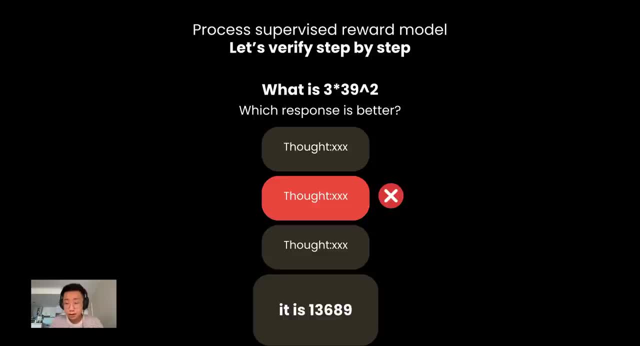 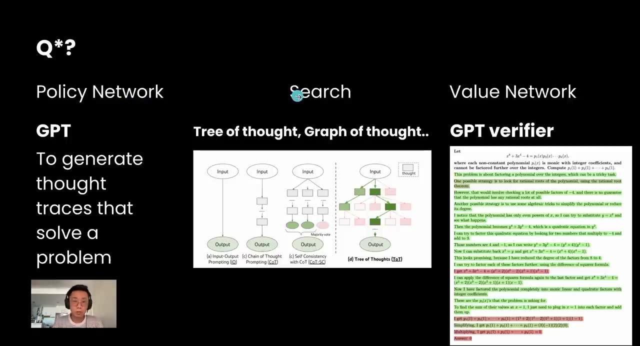 seem to lead to a much better results, which kind of makes sense, as a large range model can get a faster and more detailed feedback. So the key hypothesis is whether OpenAI figured out a way to mimic similar architecture to significantly improve GPT's reasoning and logic power. 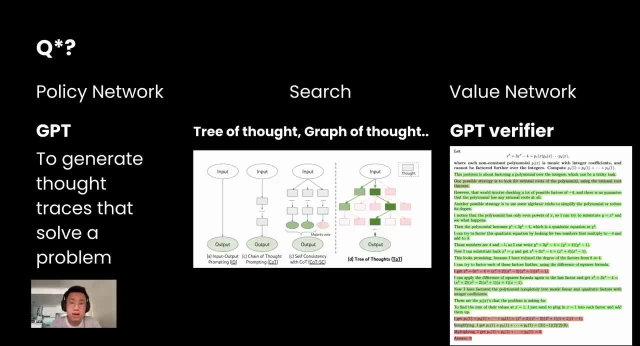 and enable it to explore strategy and problem-solving methods. that is not solved yet, But again, those are all just hypothesis and guess. There's no real concrete answer about what a Q star really is, but it's definitely useful to get a better understanding. 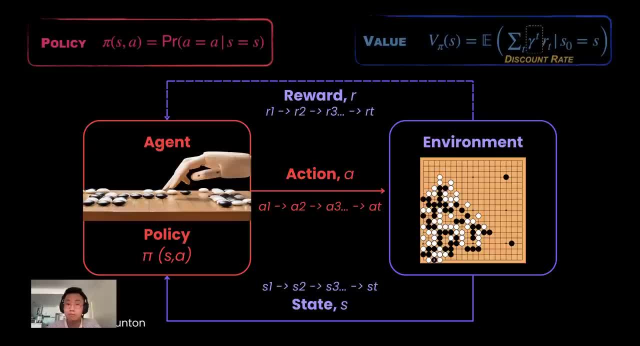 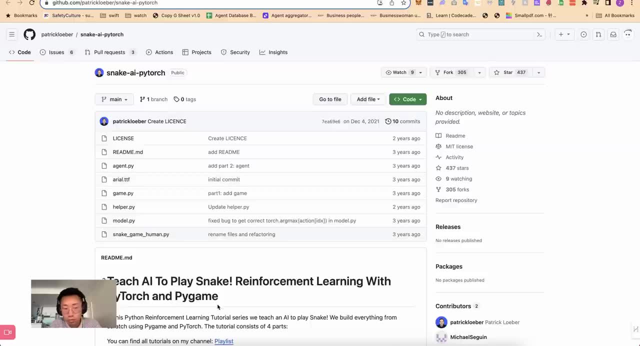 about this reinforced learning model because that really draw a different picture about how the future can look like with AI. It might sound stunning but it's actually not that hard to getting started- This open source project from Patrick where you can spin up a reinforced learning AI. 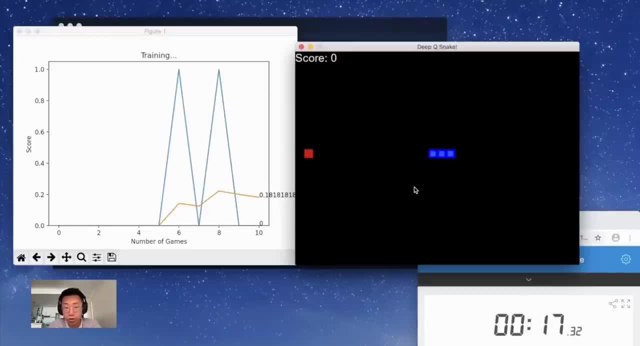 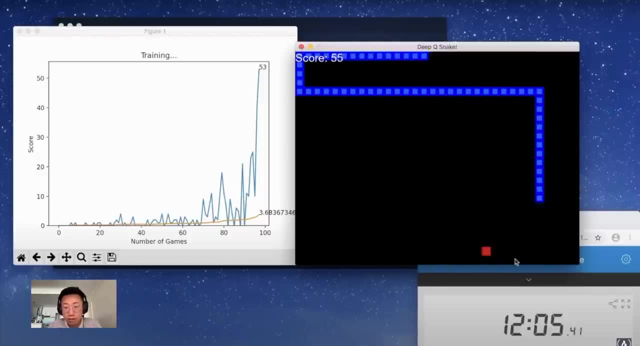 to learn how to play a snake game where, at the beginning, it has no idea about what the rules of game is, And after a few hundreds rounds of learning and testing it can achieve the same level of a pro human player, And the whole project takes less than 400 lines of code. 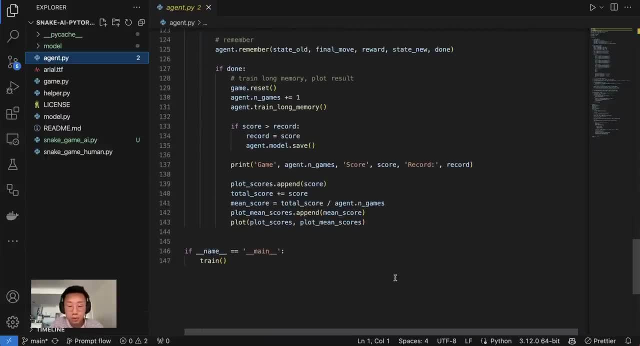 So I definitely recommend you go and try out. I'll put a link in the description below. So this is today's video. I'm really curious to hear what Q star actually is after some open AI announcement. Comment below if you have any other information. 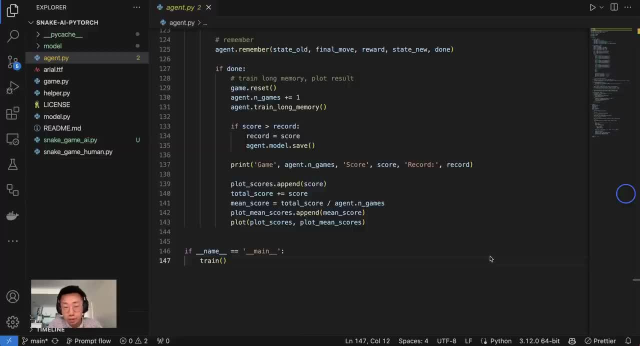 I will continue posting interesting AI projects and learnings I got, So please consider giving me a subscribe if you enjoy this content. Thank you, and I'll see you next time.